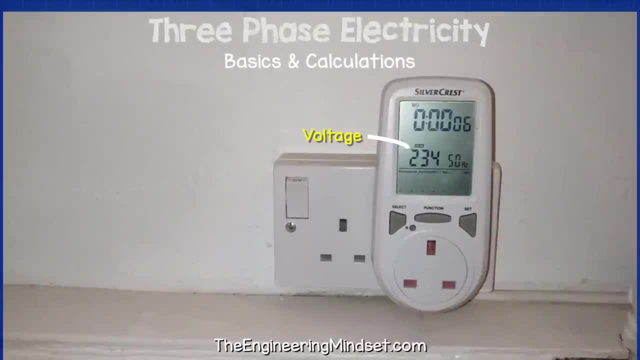 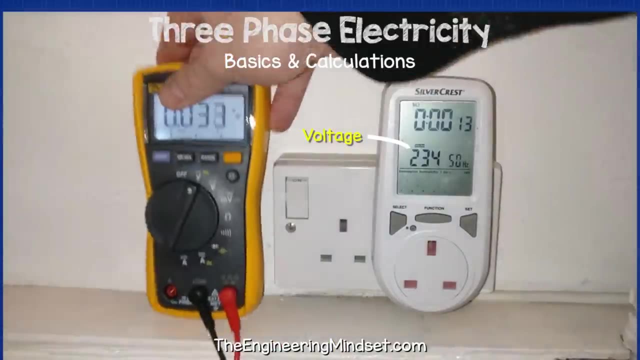 monitor. In this case it reads about 234 volts. It's lower because there are some losses in the wire, but it's not a big deal. But also the voltage varies throughout the day. Alternatively, I can also use a multimeter to take a measurement of this. I can put the probes into the socket and take a reading. 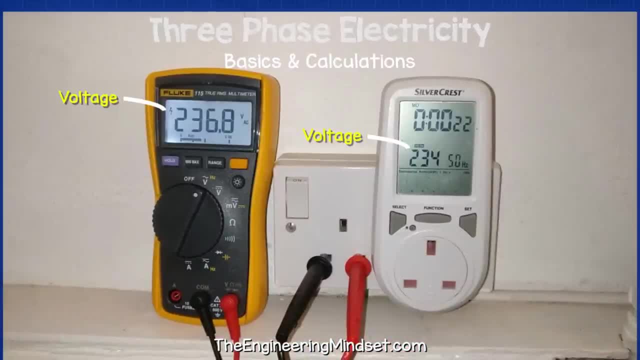 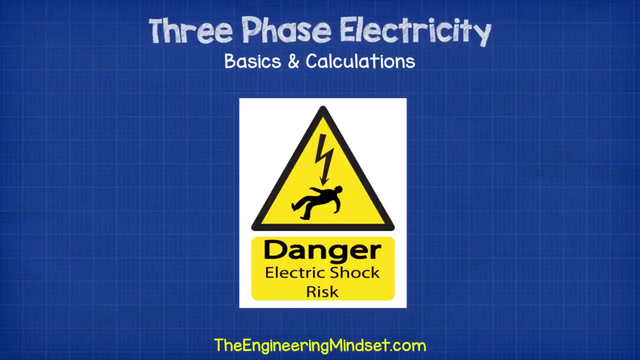 of 236.8 volts. The readings are slightly different because the multimeter is more accurate. You should be electrically competent and qualified to do this. Remember, electricity is dangerous and it can kill you If you don't have an energy meter or a multimeter. these are very 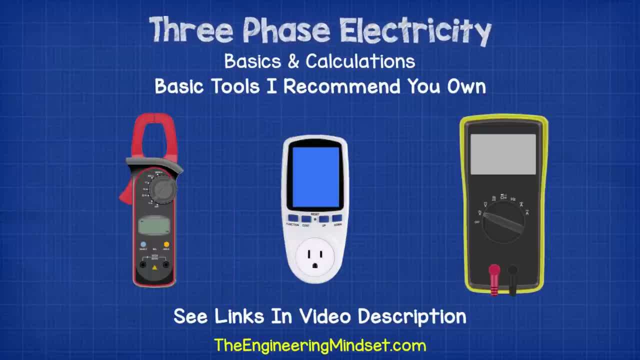 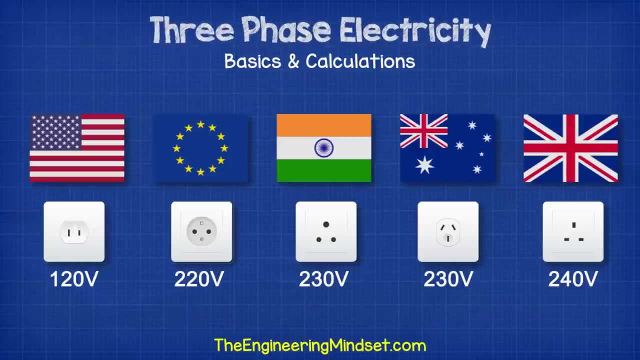 cheap and very useful. so I do recommend you get one and I'll leave a link in the video description below for where you can pick one up online for cheap. As I said, the voltages at our sockets do vary throughout the day. You can see here. I've 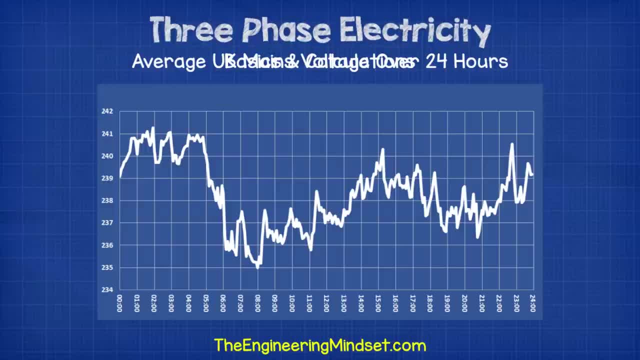 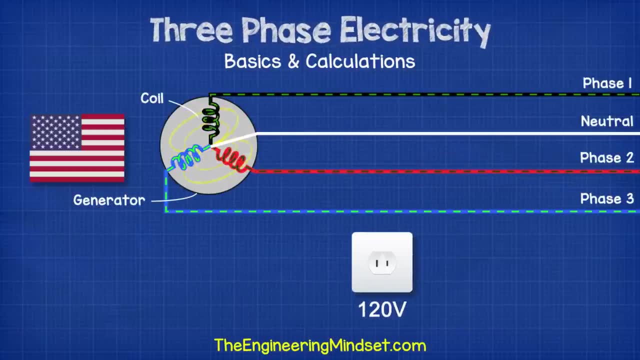 logged the average voltage every 5 minutes for 24 hours and it varied between 235 volts and 241 volts. Now these voltages at the sockets are single phase from a wire connection, from either a generator or a transformer. They come from connecting between a single phase. 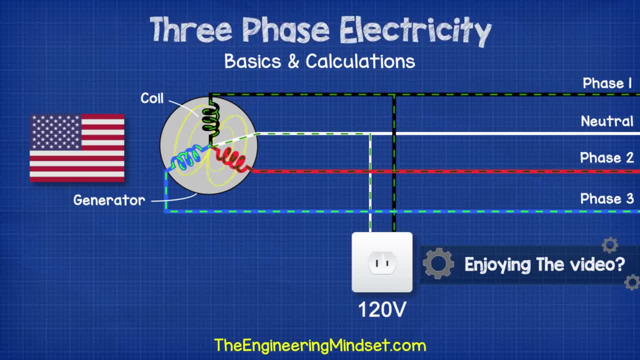 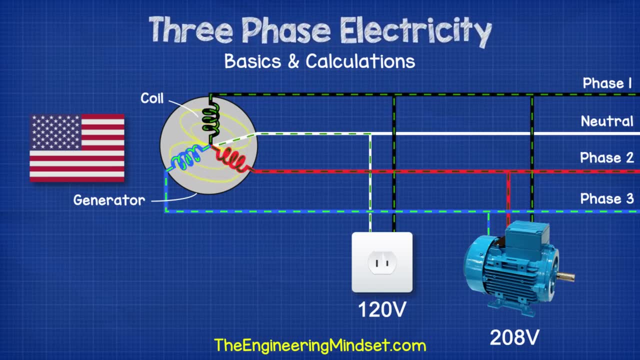 and the neutral line, or in other words, just one coil of the generator, But we can also connect to two of them. You can connect to two or three phases at once, so two or three coils of the generator. This is typical in large properties with large equipment and large appliances which need. 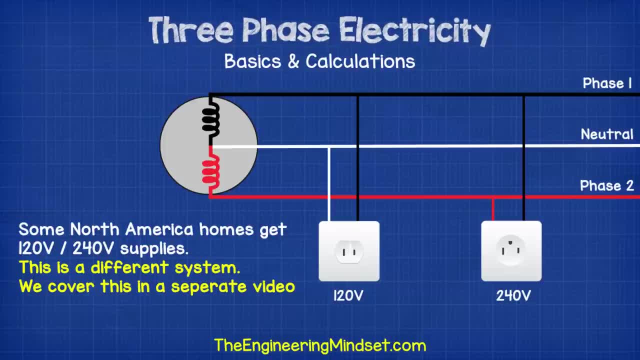 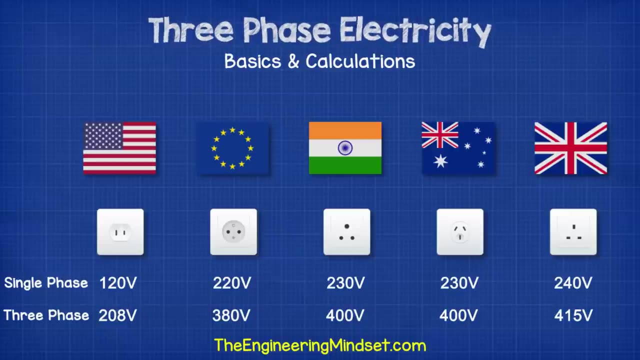 more power. In North America you often find two phase supplies in homes with 120 or 240 volts. That is a completely different system and we'll cover that in a separate video. This video is only for three phase. Looking at the different voltages in the US, we get 120 volts from a single phase or 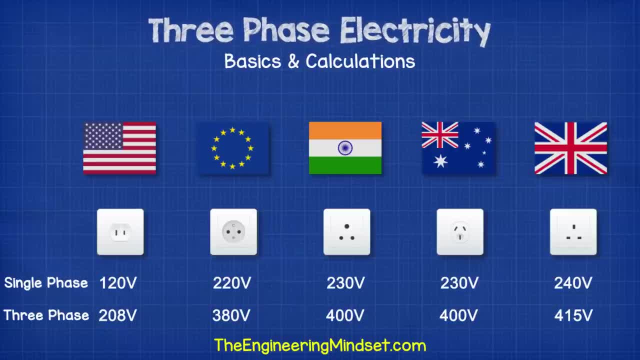 208 volts from three phases. You can also connect to two or three phases at once. This is typical in large properties with two or three phases. You can also connect to two or three phases. You can also connect to two or three phases. You can also connect to two or three phases. In Europe we get 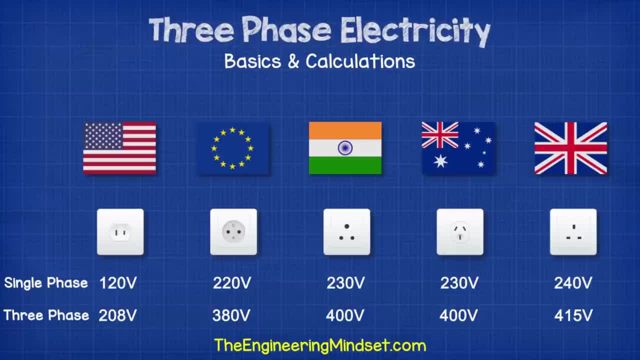 220 volts single phase or 380 volts three phase. Australia and India get 230 volts single phase or 400 volts three phase, and in the UK we get 240 Volts single phase or 415 three phase. Again, these voltages vary slightly throughout the day and it's unlikely that they will. 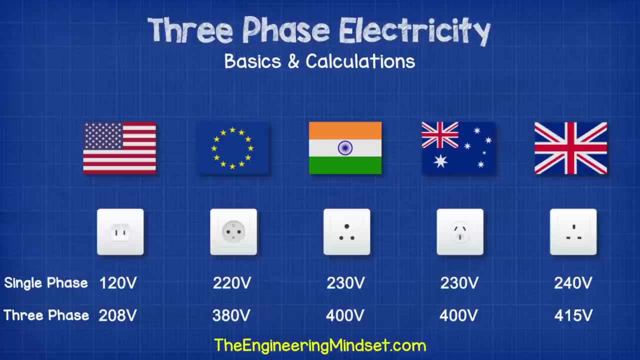 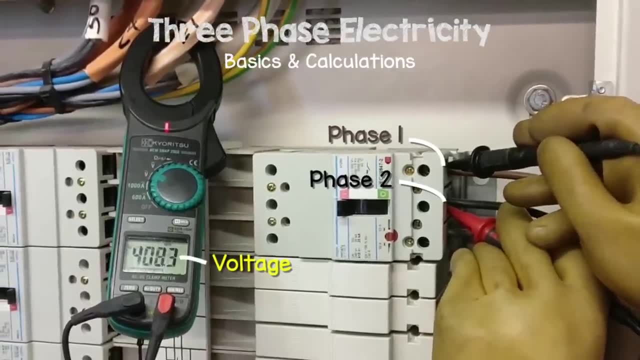 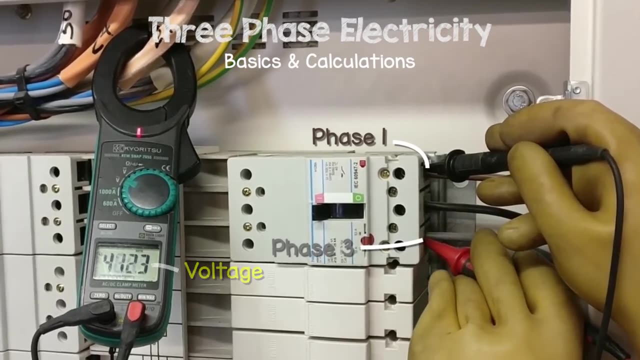 be exactly this value. We can measure the voltages in the three phase supply also. You see, here I have a three phase supply going into this breaker. If I use this clamp meter to measure between phase one and two, I get a reading of 408 volts. If I connect across phase one and phase three, I get almost. 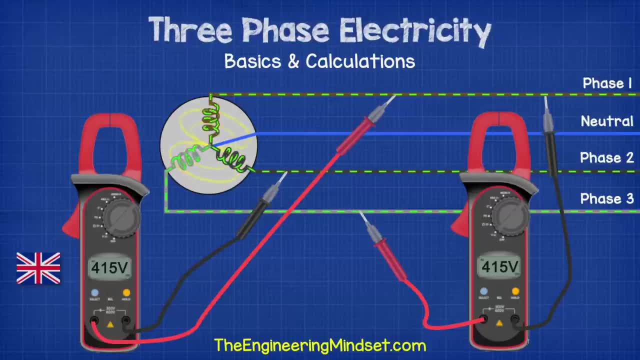 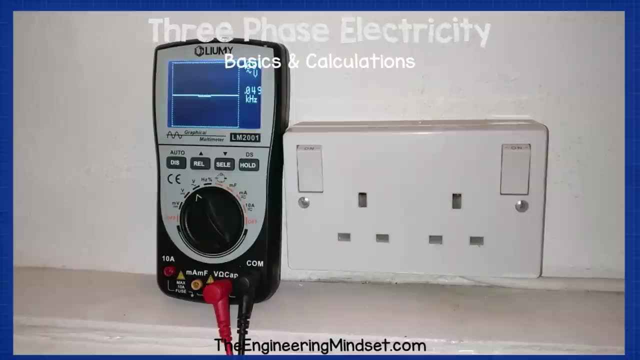 the same reading of 410 volts. So I'm reading across these two phases to get these readings. You can measure between any two of the three phases and get the same results If I use this multimeter with an inbuilt oscilloscope and connect the terminals to a single phase and neutral you. 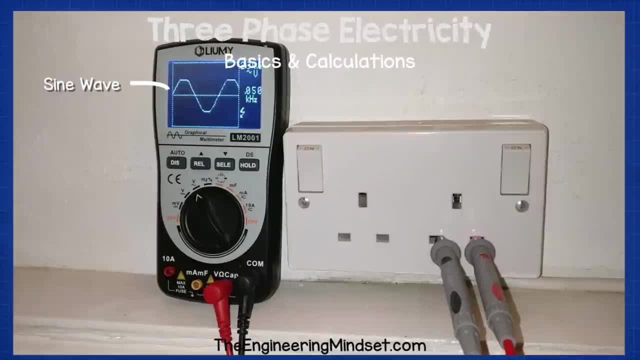 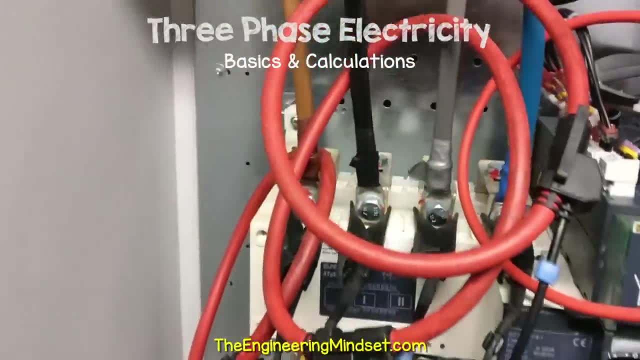 see I get a single sine wave. All three phases are producing a sine wave just at a different time. We can see this if I connect my power analyzer to the three-phase system. Here I connect to all three phases and you see, it produces these three separate sine waves, all one after another. 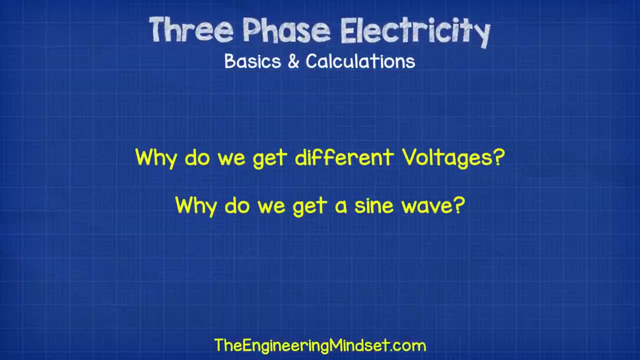 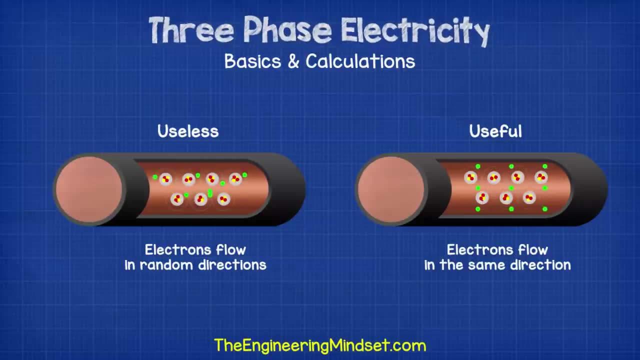 Hopefully you can see that the yellow phase is a little hard to make out. So what's happening here? Why do we get different voltages and what do these sine waves mean? So just to recap, we get useful electricity when lots of electrons move along a cable in the same direction. We use copper wires. 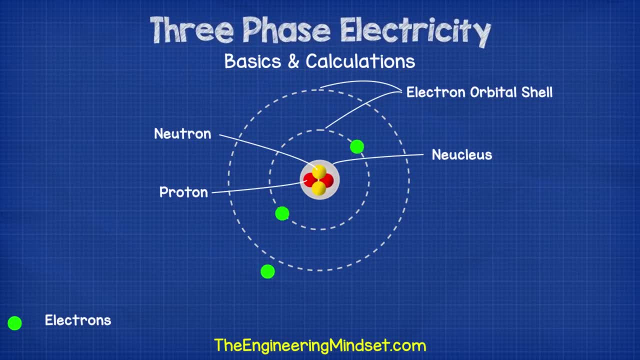 because each of the billions of atoms inside the copper material have a loosely bound electron in their outermost shell. This loosely bound electron is free to move between other copper atoms, and they do actually move all the time, but in random directions, which is of no use. 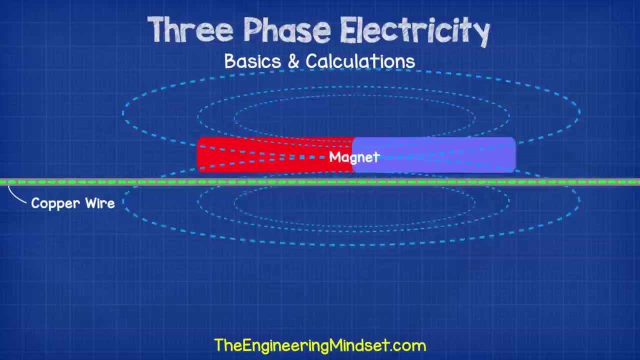 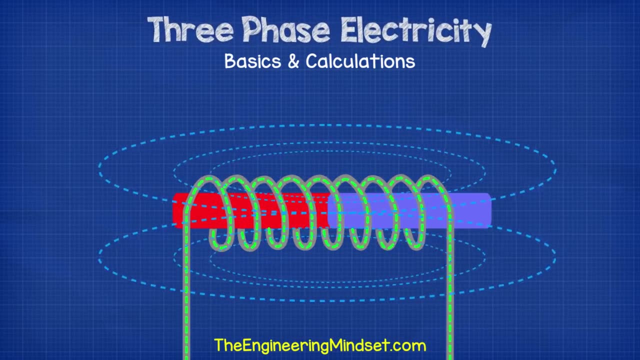 to us, So to make them move in the same direction. we move a magnet past the copper wire. The magnetic field causes the three electrons to move in the same direction. If we wrap the copper wire into a coil, we can fit more copper atoms into the magnetic field and we can therefore move more. 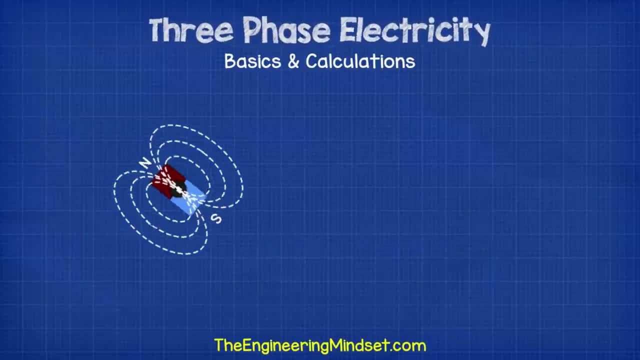 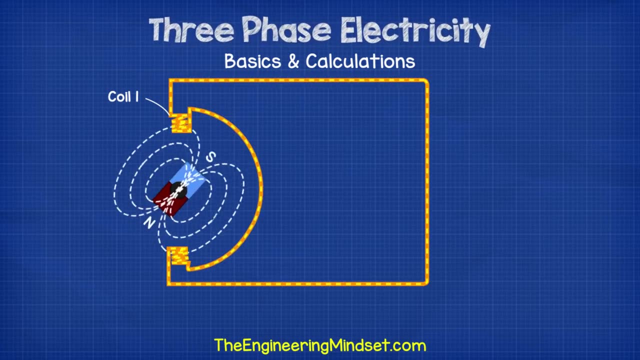 electrons. This gives us an alternating current Instead of someone moving a magnet. we can move a magnet back and forth all day. Engineers instead just rotate it and then place a coil of copper wire around the outside. We split the coil into two, but keep them connected, and then place one at the top. 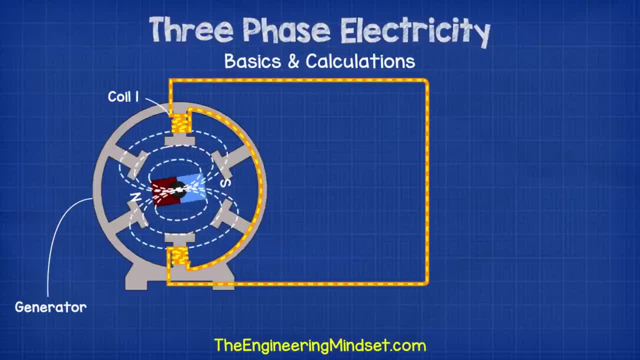 and one at the bottom to cover the magnetic field. When the generator starts, the north and south pole of the magnet are directly between the coils, so the coil doesn't experience any effect and no electrons move. As we slowly rotate the magnet, the north side passes the top coil and this pushes 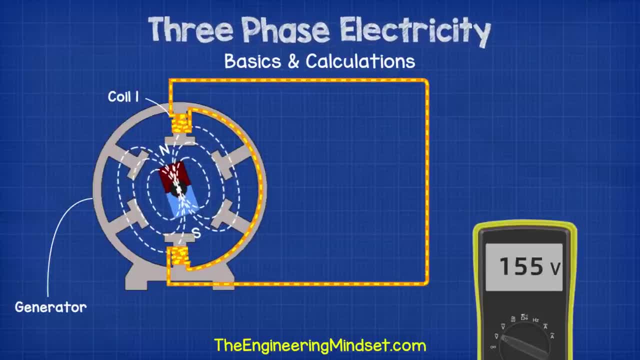 the electrons forward, so we get positive values. The strength of the magnetic field increases as it rotates up to its maximum, where the most electrons are flowing. The magnetic field then starts to decrease and less electrons flow until the magnet is again directly between the two coils. Then the south pole rotates in, but this 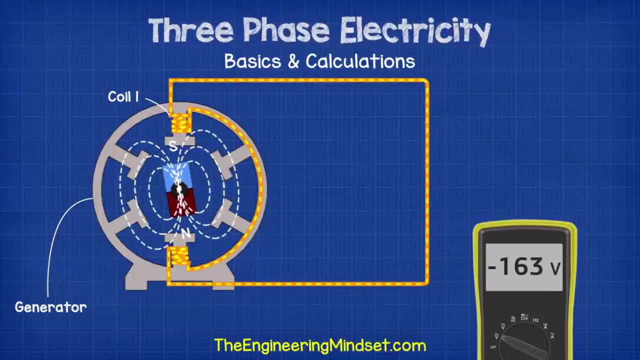 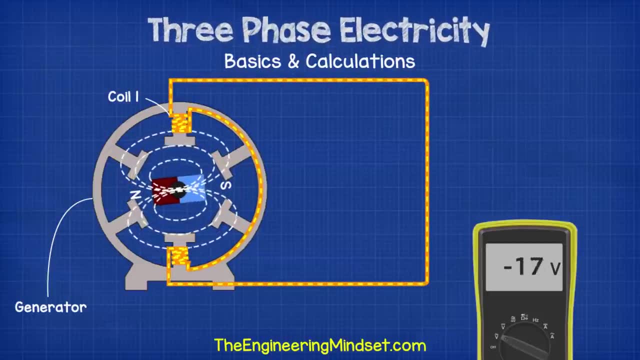 time it pulls the electrons backwards, so we get negative values. This again increases in strength up to its maximum and then decreases back to zero where the magnet is between the two coils. If we plot these values then we get a sine wave. The north side. 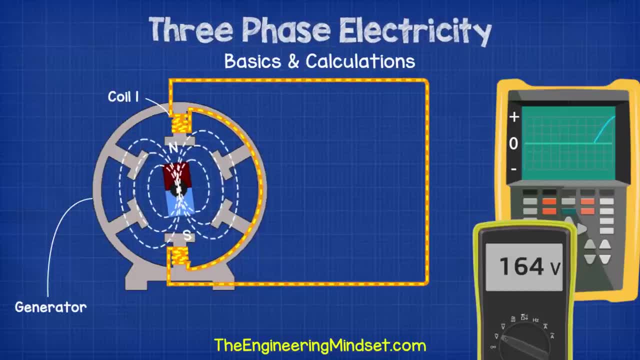 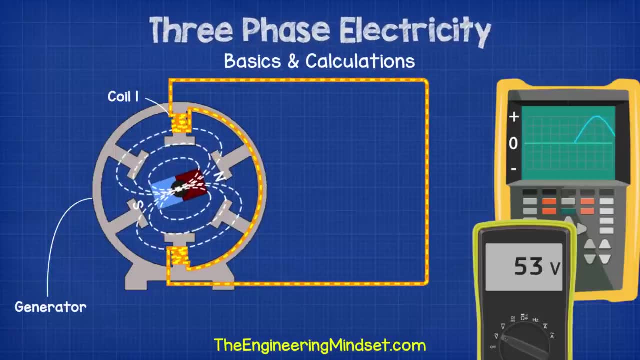 pushes the electrons forward and as the strength of the magnetic field increases, more electrons flow up to a maximum point. Then we're leaving the north magnetic field, so the number of electrons decreases down to zero. Then the south pole pulls the electrons backwards, so we get the negative. 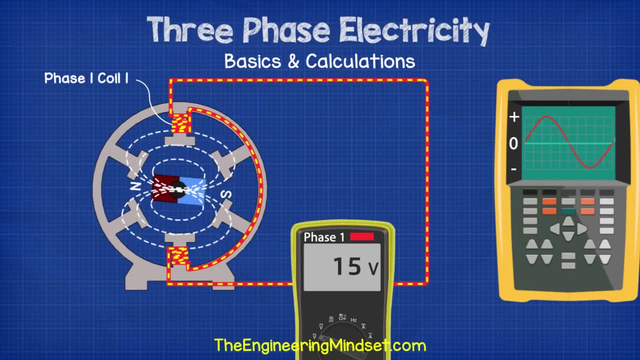 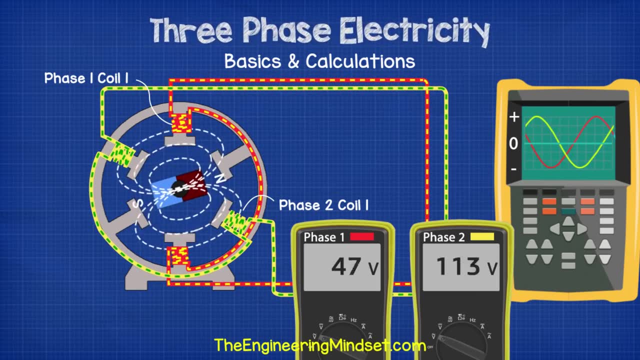 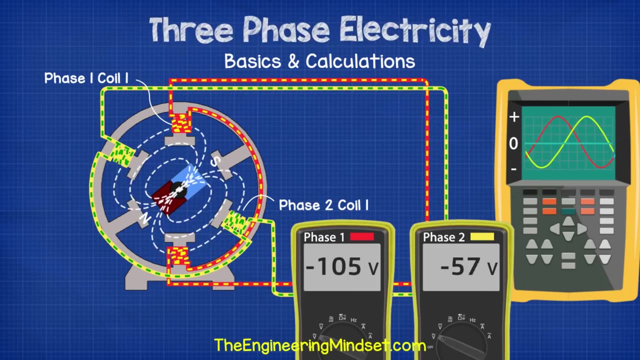 values up to a maximum and then back to zero. This one circuit gives us a single phase supply. If we added a second coil, set 120 degrees rotation from the first, then we get a second phase. This coil will experience the change in magnetic field at different times compared to the first phase. 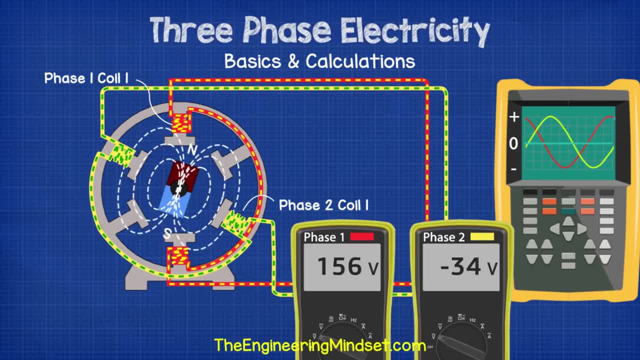 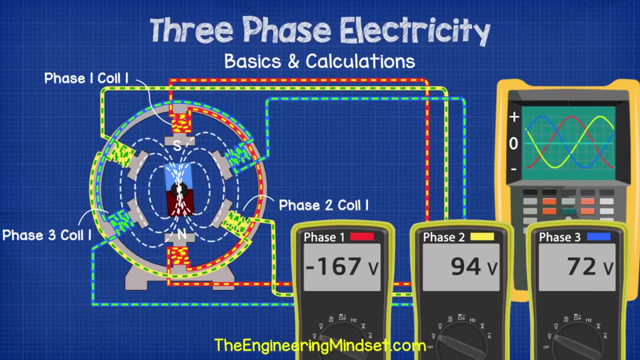 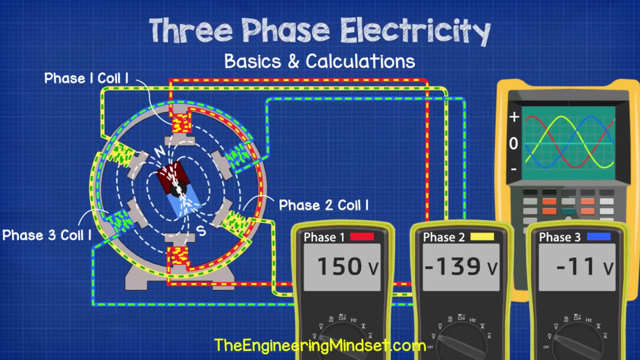 So its waveform will be the same, but it will be delayed. The second phase waveform doesn't start until the magnet rotates to 120 degrees rotation. If we then add a third coil, 240 degrees rotation from the first one, then we get a third phase Again. this coil will experience the change in. 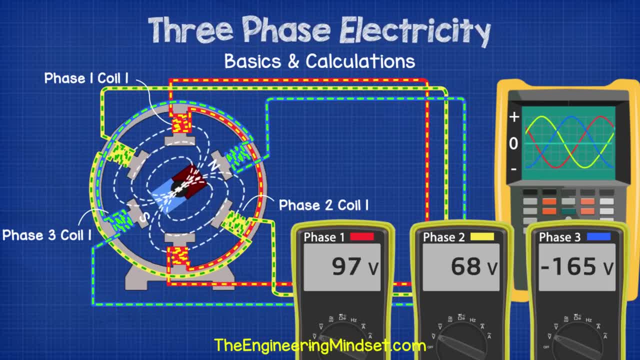 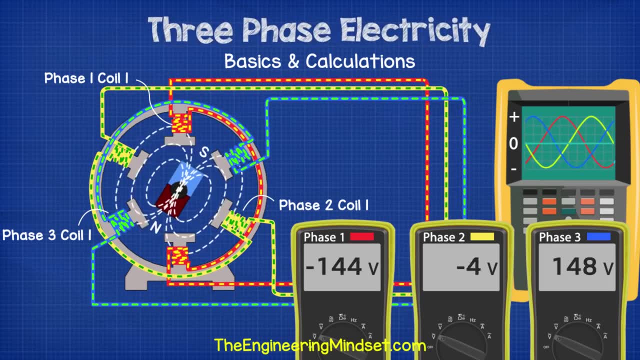 magnetic field at a different time to the other two, So its wave will be equal to the others, except it will be further delayed and will start at 240 degrees rotation. When the magnet rotates multiple times it eventually just forms an unbroken three phase supply with these three waveforms. 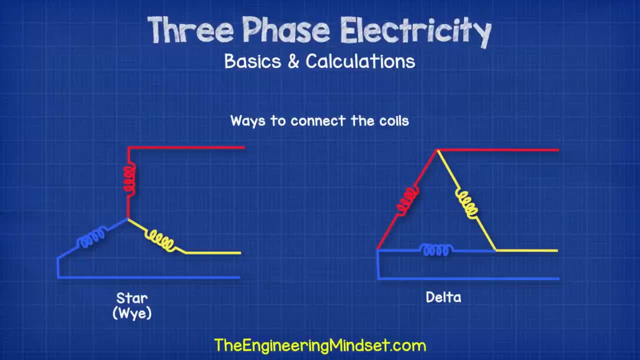 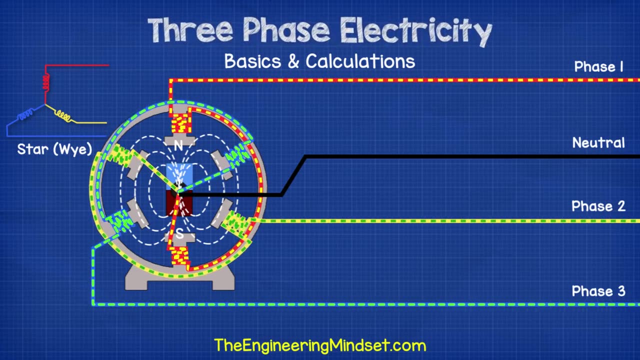 With this design we need six cables, But we can join them together in either a delta or y method. For this example, I'm going to use a y or star method because I think it's easier to understand With a star configuration. we need just four cables: One for each of the three phases and then a neutral. 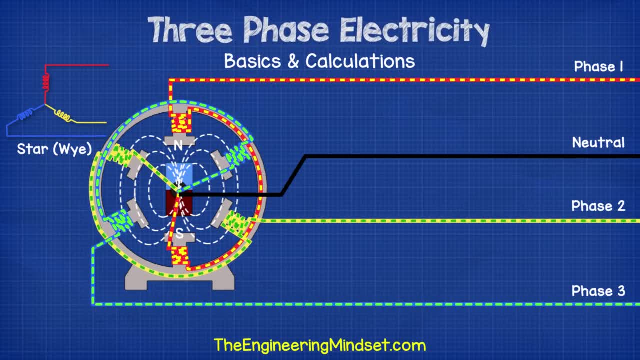 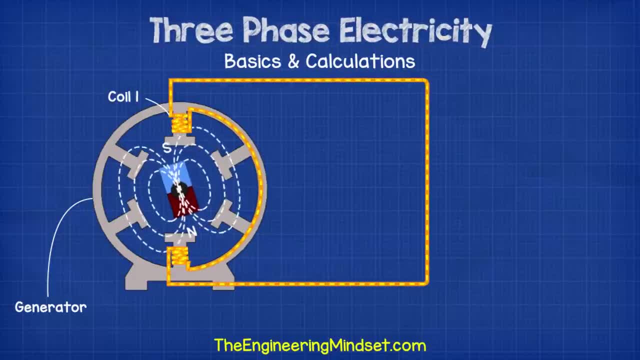 When the magnet completes one third of the phase supply, then we get a second coil. When the magnet completes one third of the phase supply, then we get a second coil. Now let's slowly rotate the generator and calculate the voltages which cause the sine wave. 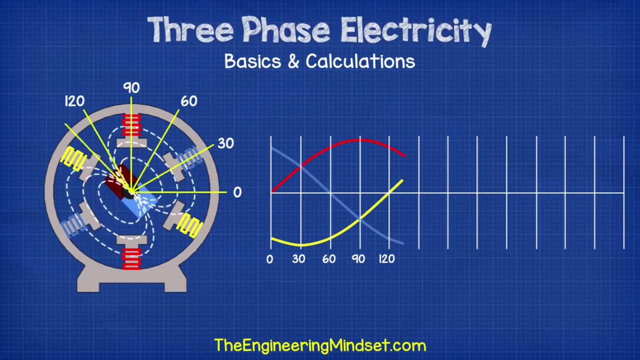 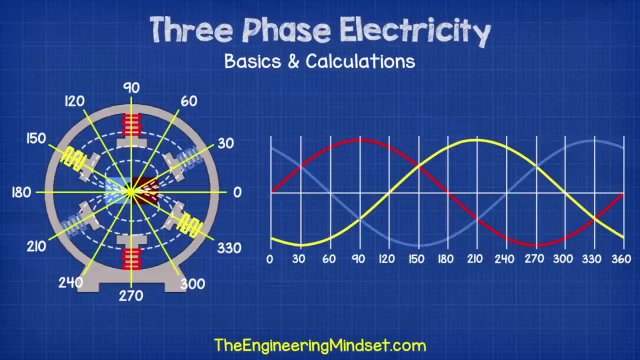 for each of the three phases. Let's first divide the rotation up into segments, 30 degrees apart, giving us 12 segments. We'll cover the instantaneous voltage at each of these rotation points for each of the three phases. Now I'm using Excel to calculate these. 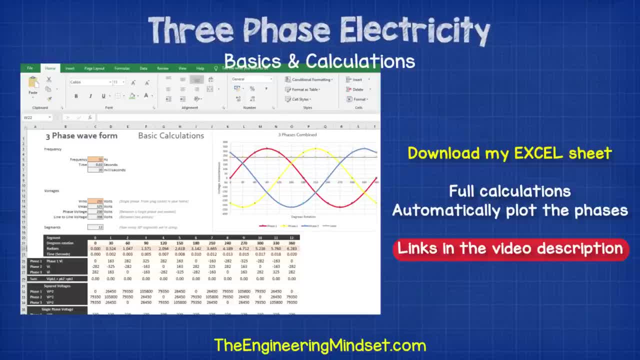 and if you want a copy of my Excel sheet with all the calculations in, then I'll leave some download links in the video description below For the video worked example: I'm going to use 120 volts VRMS. The sheet will update itself. 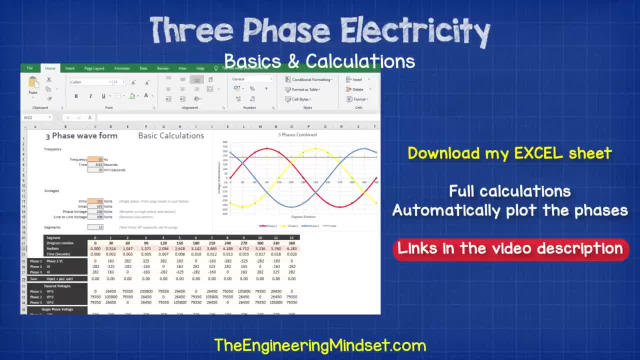 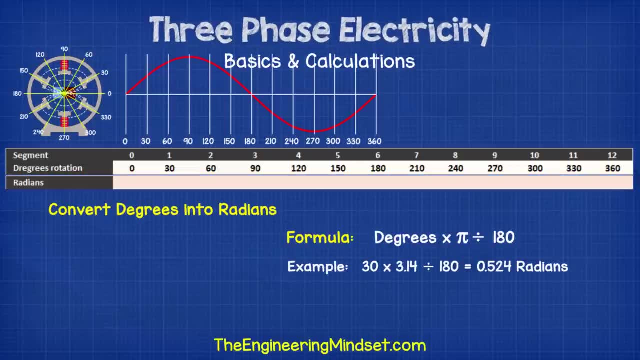 plot the phase waveforms and give you the calculations Again. links down below for that. So we first write out a table showing each of the segments and then the angle of rotation in degrees. First we need to convert each segment from degrees into radians. 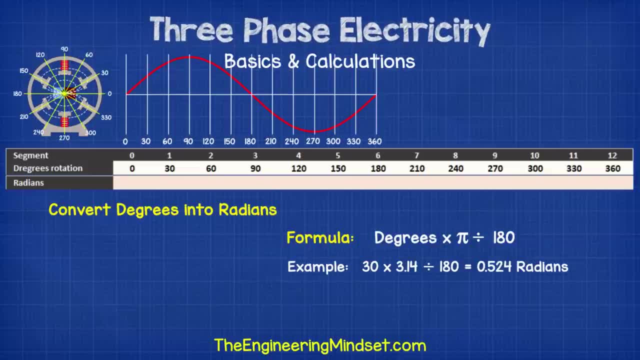 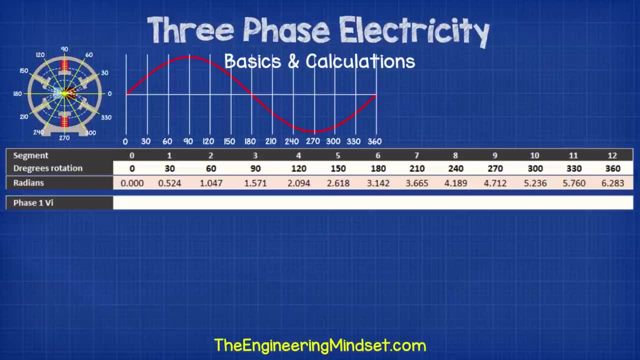 We do that by using the formula radians equals degrees multiplied by pi, divided by 180.. So we calculate the radian value for each segment and fill in the chart. Now we want to calculate the instantaneous voltage at each of these 30 degrees. We calculate the instantaneous voltage. 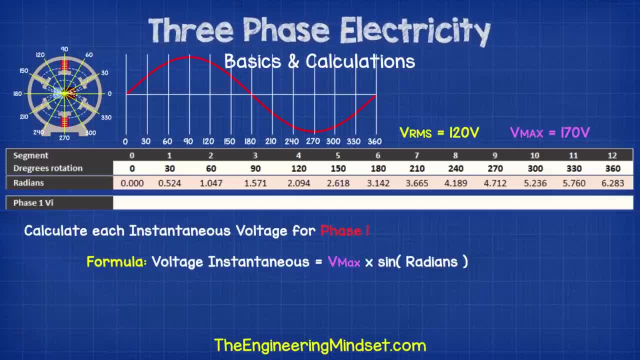 at each segment using the formula Vmax multiplied by sin angling radians. As I said, for this example we'll be using 120 volts of RMS and, as we calculated earlier, that gives us a Vmax of 170 volts. So just complete that calculation for each segment. 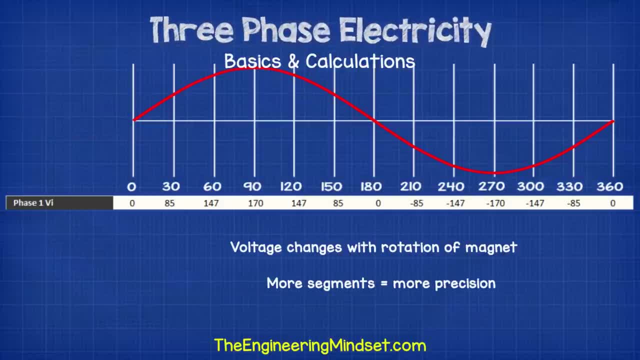 until the table is complete for one full cycle. Now if we plot this, then we get a sine wave showing the voltage at each point during the rotation. You can see now how the voltages increases with the rotation. So if we plot this, then we get a sine wave. 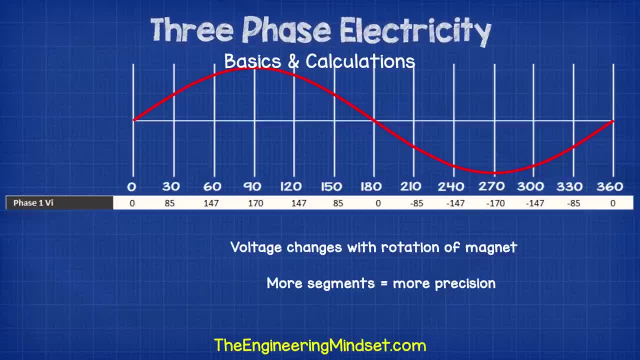 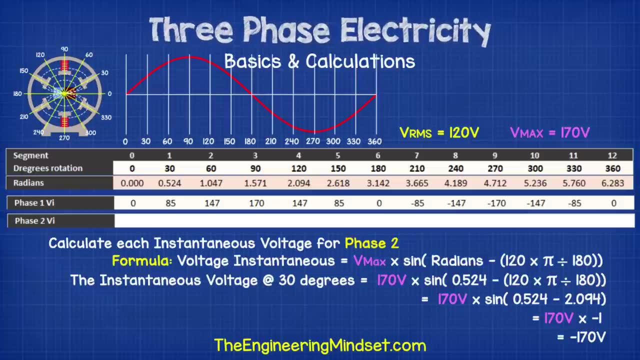 showing the rotation of the magnet. and when the polarity of the magnet changes, the voltages become negative. Now we can calculate phase two voltages and we can do that using the formula Vmax multiplied by sin, angling radians minus 120 times pi divided by 180. 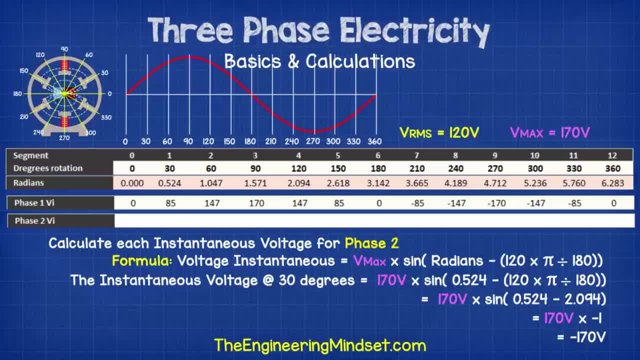 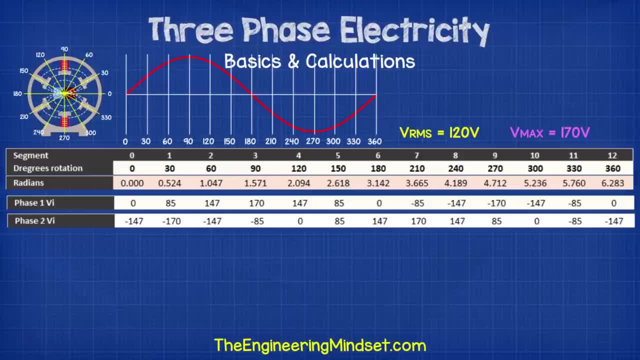 This end part, 120 times pi divided by 180, just takes into account the delay, because the coil is 120 degrees from the first one, and then it converts this to radians. So we can now plot this for each segment until the table is complete for one full cycle. 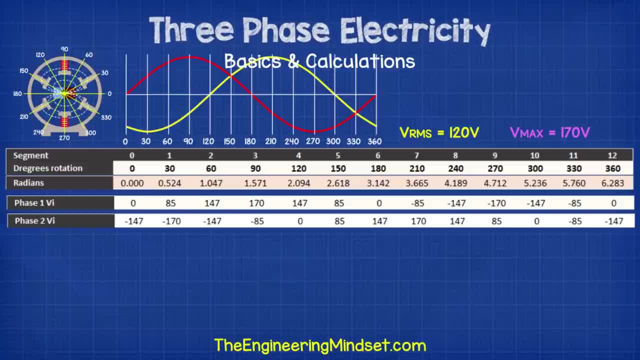 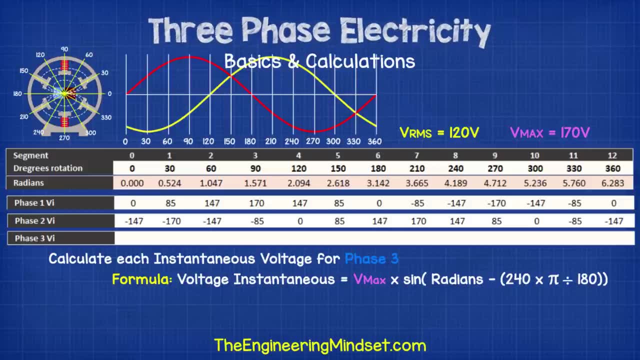 We can now plot this to see the waveform for phase one and two and how these voltages are changing. For phase three we need to use the formula Vmax multiplied by sin angling radians minus 240 times pi divided by 180.. 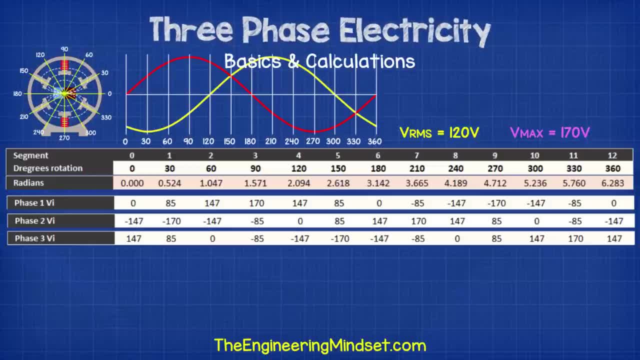 So just complete that calculation for each segment until the table is complete for one full cycle. We can now plot this to see the waveform for phases one, two and three and how the voltages are changing. So this is our three-phase supply showing the voltage. 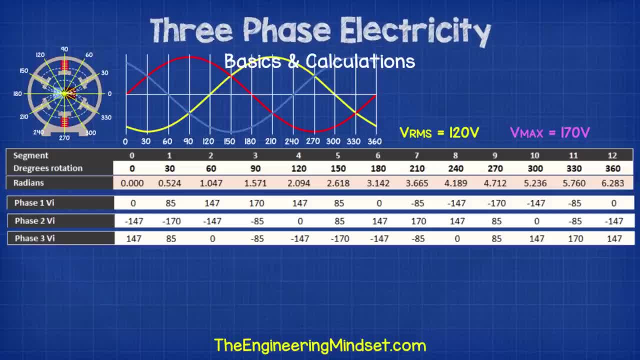 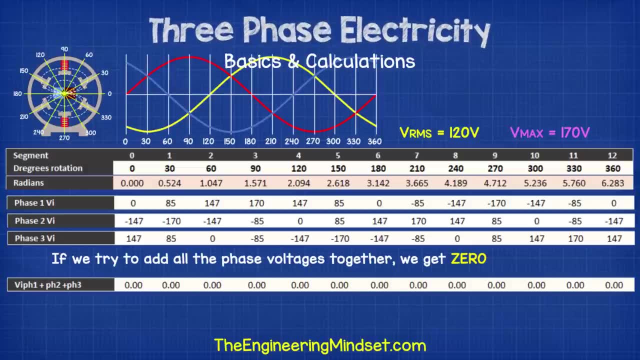 for each phase every 30 degrees rotation of the generator. If we try to add these voltages together, we get zero because they cancel each other out. So instead we're going to take the RMS voltage per phase. I'll just show you this for one phase. 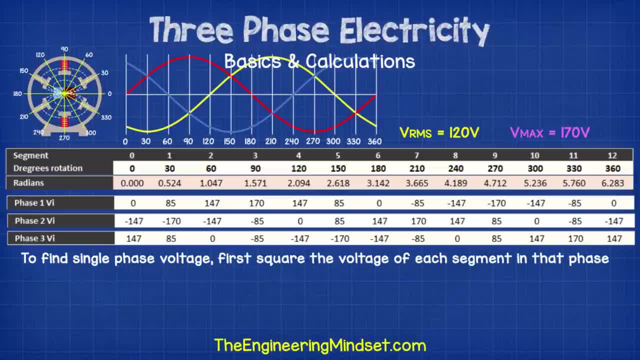 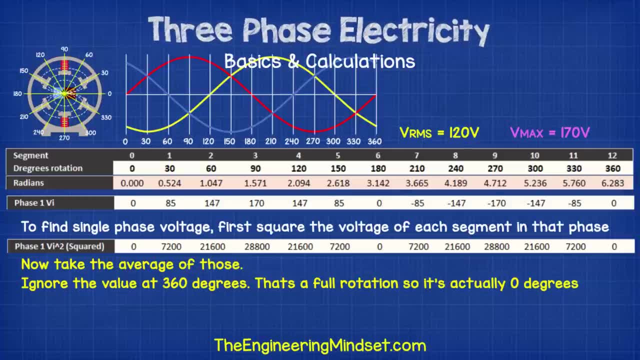 but the process is the same for phase two and three. So we start by first squaring each instantaneous voltage for a full rotation. Now take the average of these values, Add them all together and divide by how many segments you have. In this case we have 12 segments. 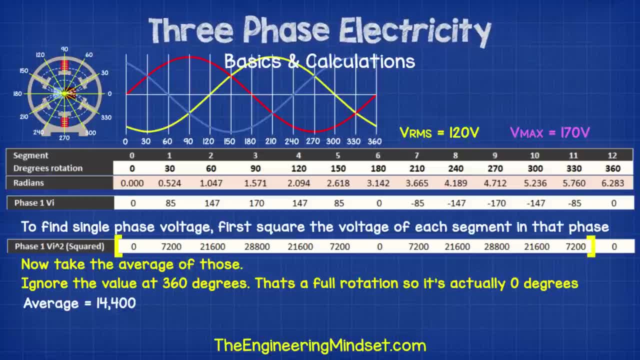 Do not include the value at 360 degrees, because this is a full rotation. so 360 degrees is back to start, which is zero. If you include this, you'll be counting the zero value twice and your calculation will be higher. Now we take the square root of that number. 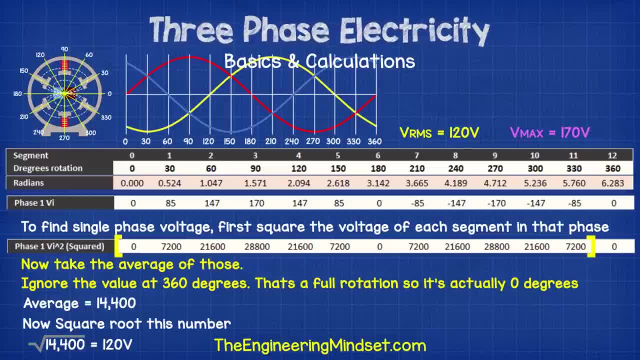 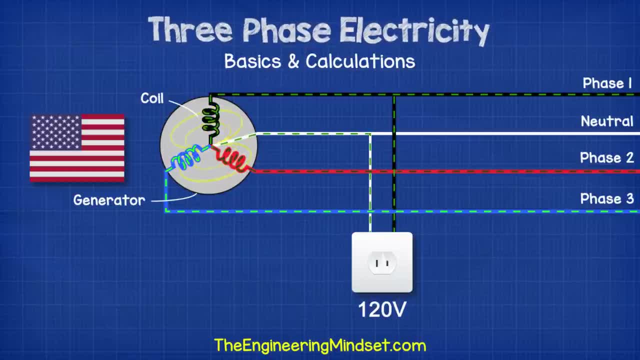 This gives us our RMS voltage of 120 volts. This is the phase voltage. That means if we connect a device between any phase and the neutral line, then we get the VRMS of 120 volts. We can do the same for phases two and three. 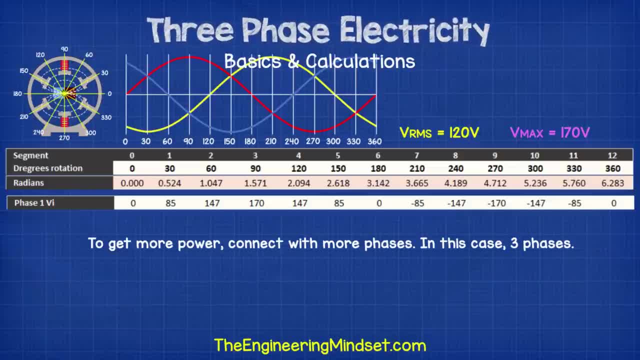 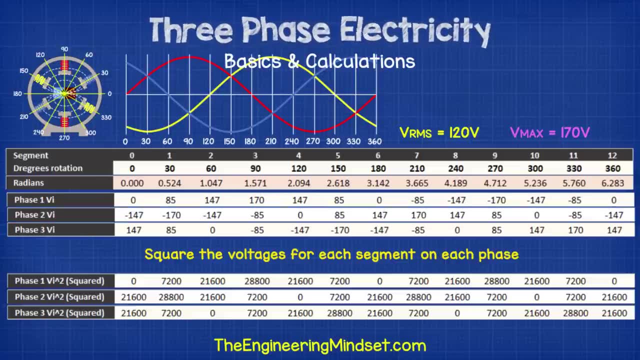 and we'll get the same value. To get more power, we can connect to all three phases. We calculate the supplied voltage by squaring each of the instantaneous voltages on all three phases. We then find the average for each phase individually and then we add these three averages together. 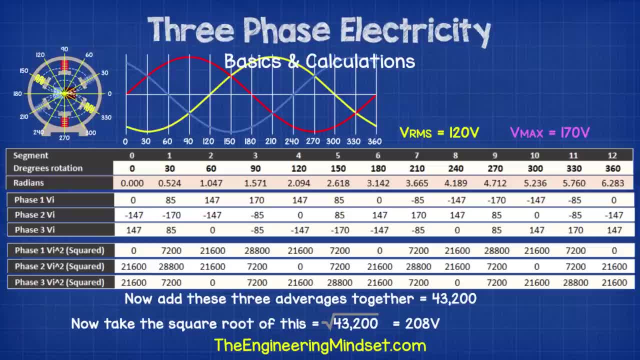 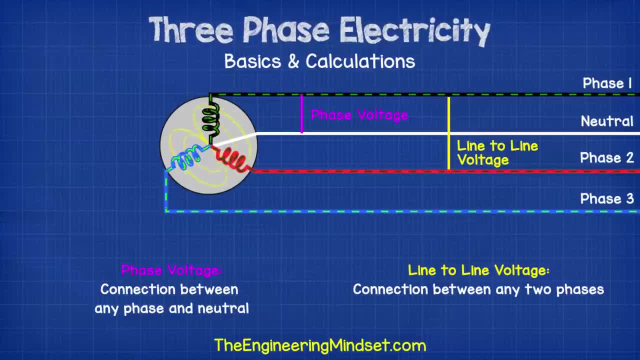 Then we take the square root of that number, You'll see the three phase voltages comes out to 208 volts. We call the smaller voltage our phase voltage and we get that by connecting between any phase and the neutral line. We call the larger voltage our line-to-line voltage. 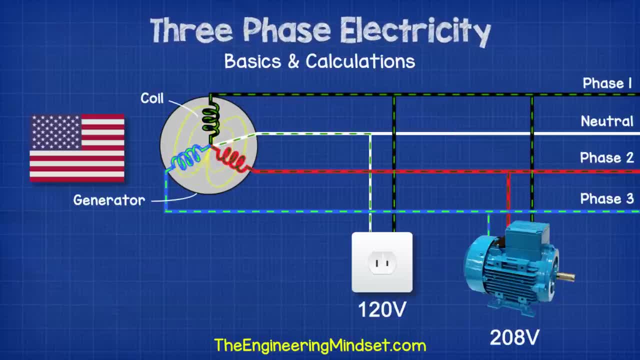 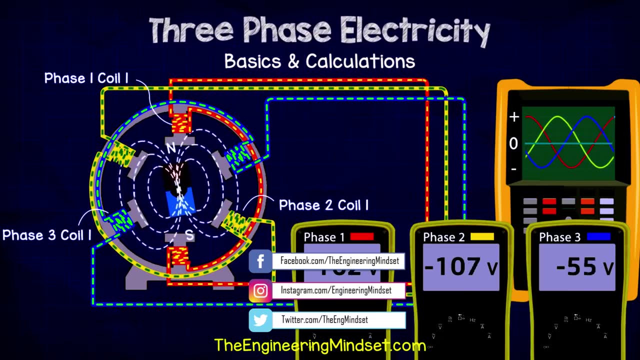 and we get that by connecting between any two phases. That's how we get more power from the supply. Okay, that's it for this video, but if you want to continue your learning, then check out one of these videos on screen now. 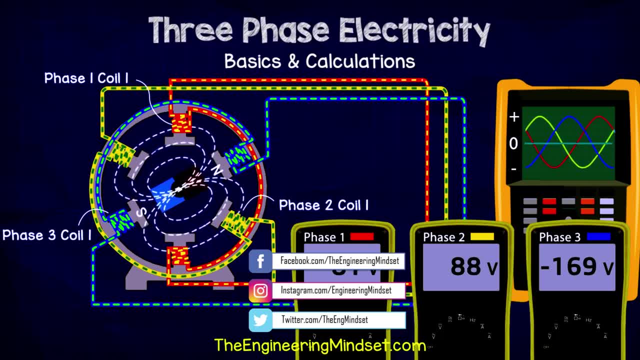 and I'll catch you there for the next lesson. Don't forget to follow us on Facebook, Twitter, Instagram and, of course, TheEngineeringMindsetcom.